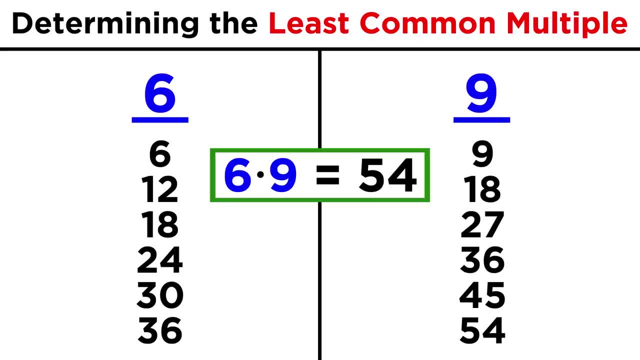 Six times nine is fifty-four. but if we write out the multiples for both numbers, we find that already at eighteen we get the least common multiple. so when looking at smaller numbers it is a good idea to write out the multiples to find the answer. 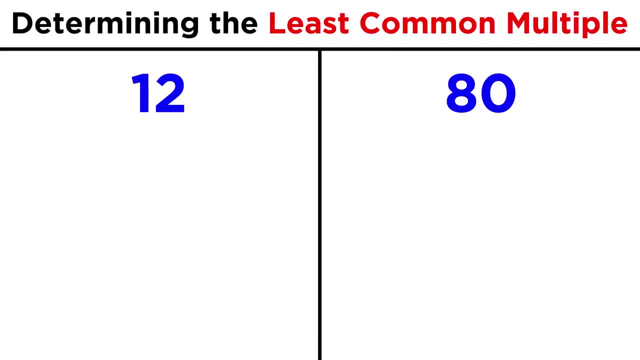 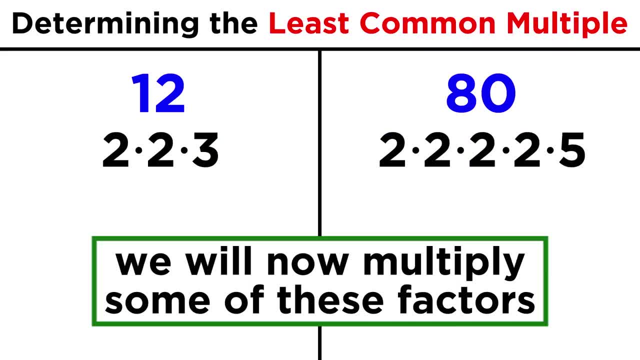 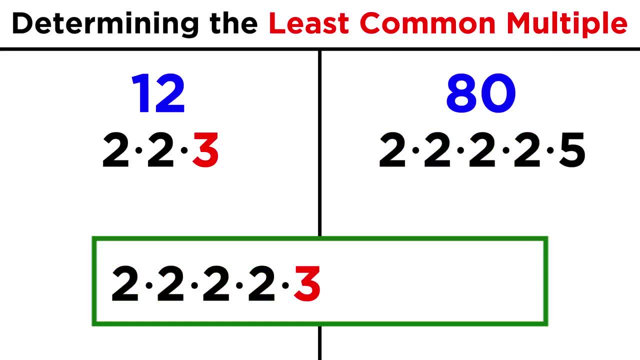 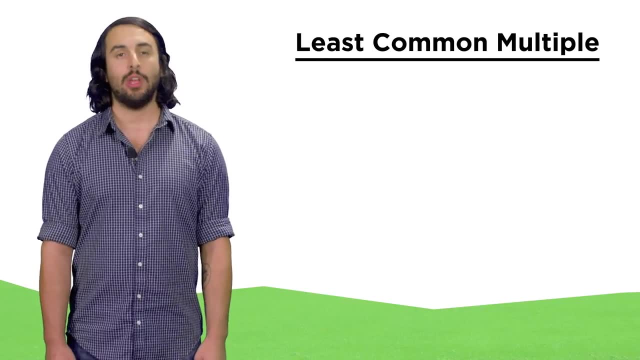 so let's put four twos, And then the one three and then the one five, We find the product and that's two hundred forty. so this will be the least common multiple for twelve and eighty. What is one application of this concept? 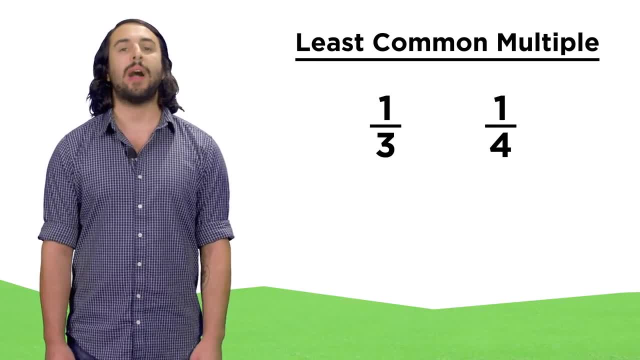 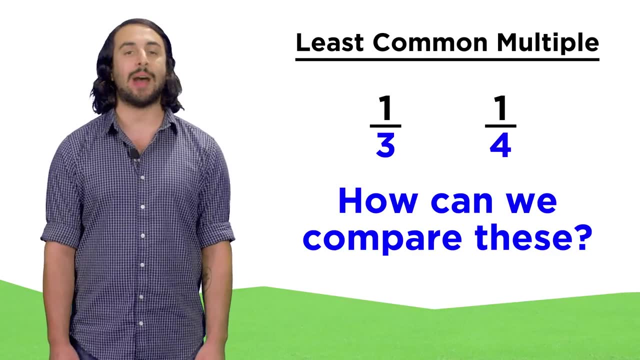 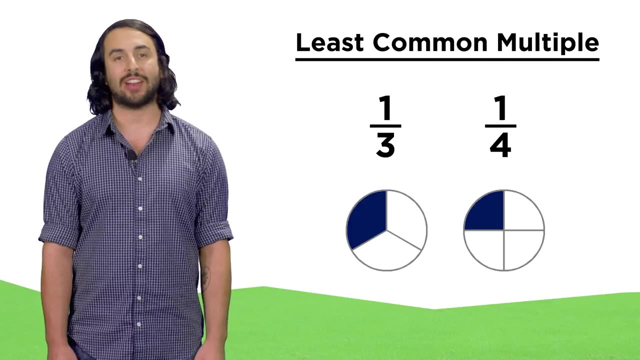 Well, we learned about fractions and sometimes we might want to know which of two fractions is larger, which can be difficult if they have different numbers in the denominator. Take one third and one fourth, for example. It's true that if we represent these fractions as sections of a circle, it is pretty easy. 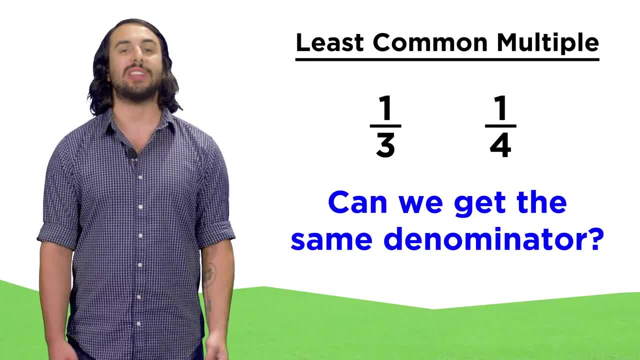 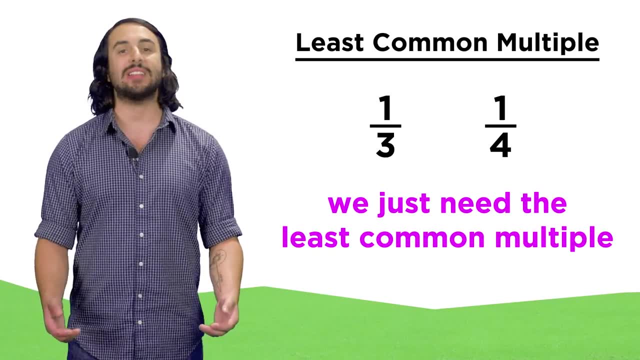 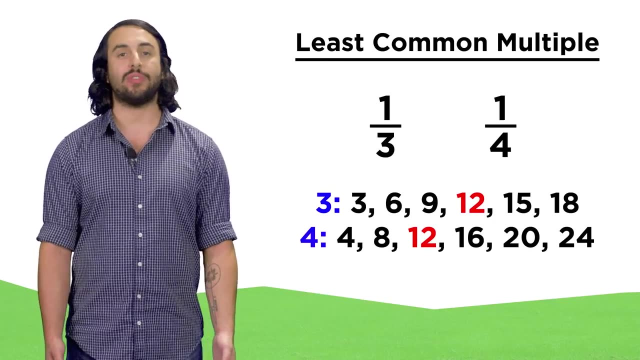 to see that one third is larger. but this becomes even more obvious if we alter these fractions so that they do have the same denominator, by finding the least common multiple For three and four. that's twelve. so what do we need to do to get twelve on the denominator? 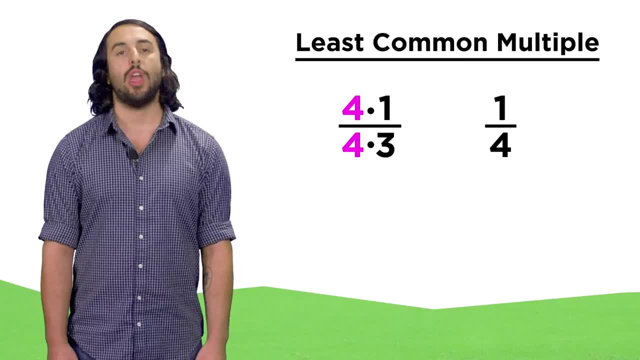 for both of these fractions For one third. we can multiply them by one third, so that's twelve. So what do we need to do to get twelve on the denominator for both of these fractions? We need to multiply both top and bottom by four.